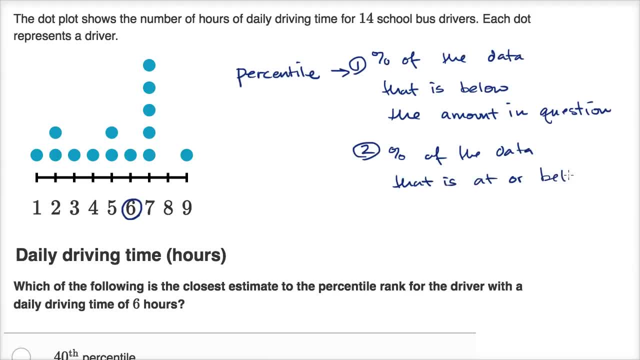 That is at or below the amount, the amount in question. So if we look at this right over here, let's just figure out how many data points, what percentage of the data points, are below six hours per day. So let's see there are. I'm just gonna count them. 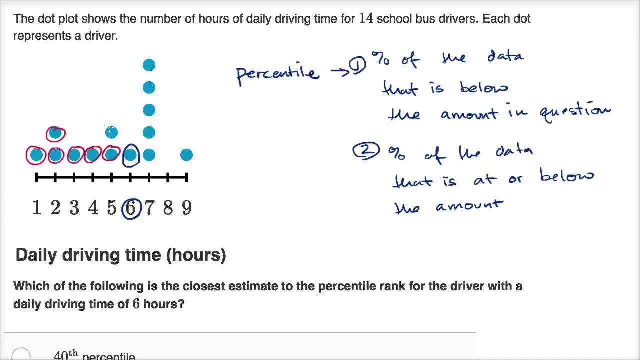 one, two, three, four, five, six, seven. So seven of the 14 are below six hours. So we could just say seven. if we use this first technique, we would have: seven of the 14 are below six hours per day. 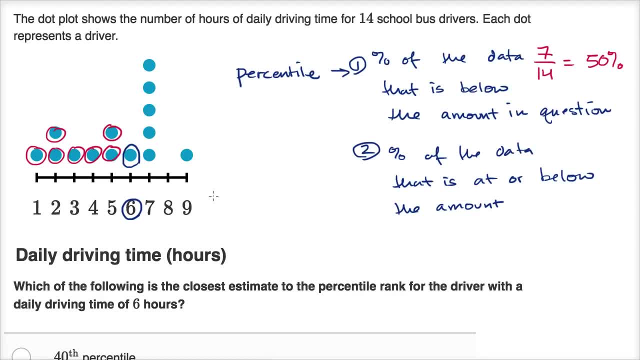 And so that would get us a number of 50%. that six hours is at the 50th percentile. If we want to say what percentage is at that number or below, then we would also count this one. So we would say eight or eight out of 14,. 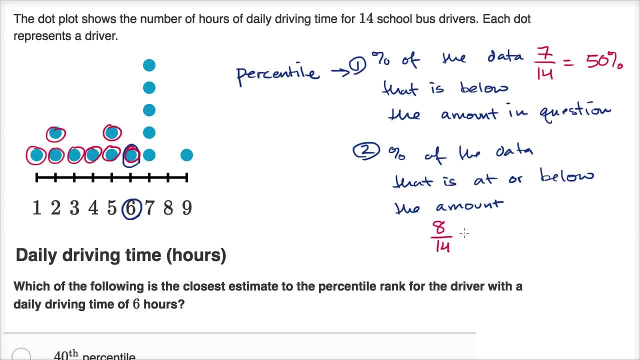 or eight out of 14.. Eight out of 14, which is the same thing as four out of seven, And if we want to write that as a decimal, let's see seven goes into four point zero, zero, zero. We just need to estimate. 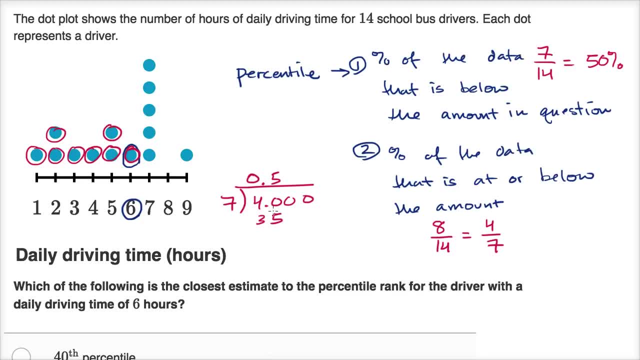 So seven goes into 40, five times 35, we subtract, we get a five, bring down a zero goes five times. look, it's just gonna be .5 repeating So 55.5555%. So either of these would actually be a legitimate response. 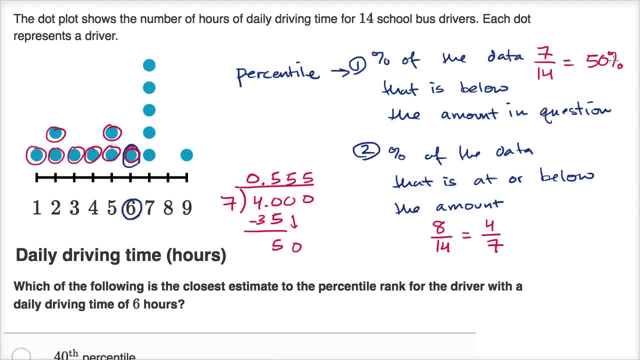 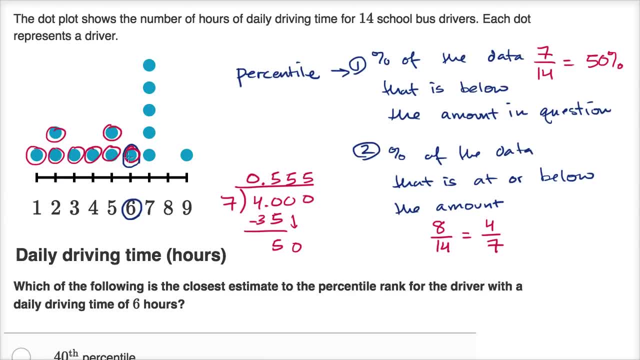 So the Kaydine gives an approximate response to the percentile rank for the driver. remarkable response to the percentile rank for the driver with the daily driving time of six hours. It depends on whether you include the six hours or not. So you could say either the 50th percentile. 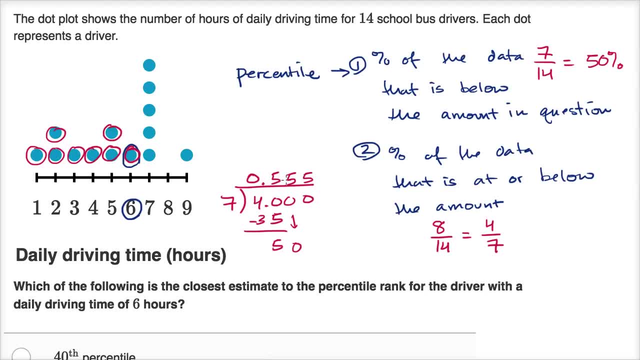 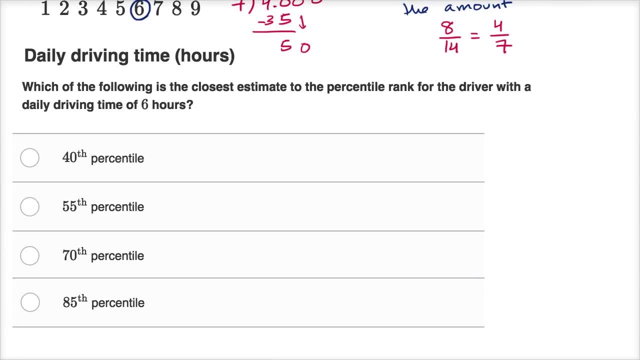 or roughly the 55th- actually the 56th percentile if you wanted to round to the newest percentile. Now, if you look at these choices here- lucky for us- there's only one choice that's reasonably close to either one of those. 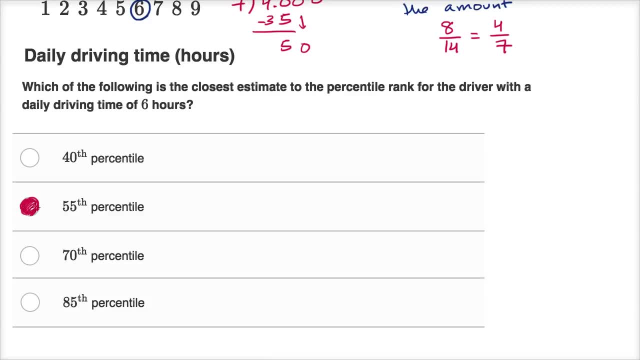 and that's the 55th percentile. It looks like the people who wrote this question where they include the data point in question. So everything at six hours or less, what percentage of the total data is that?